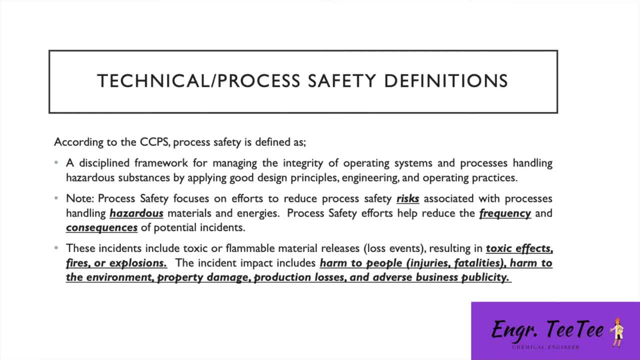 well, includes harm to people, harm to the environment, um property damage, production losses and um damage to the business reputation. so these are these. things are important. that and this, these are the. these are the reasons why process safety is very important, because we don't want people to be harmed, we don't want to harm the environment and we definitely as well don't want um bad. 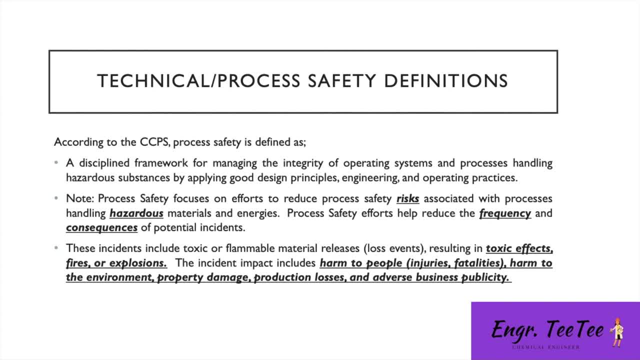 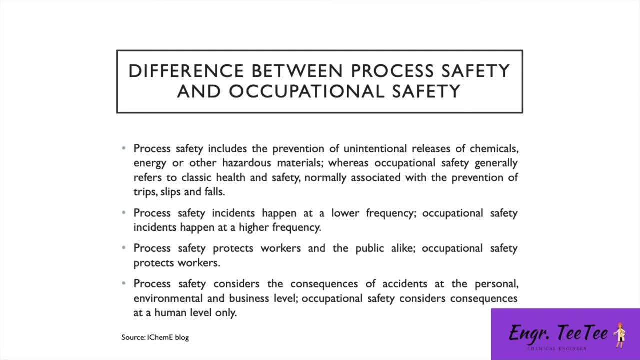 publicity or production losses as well. this is so. this is why process safety is very important. so one thing that always gets um mixed up is occupational health and safety with process safety. so this is um sourced from the ikemi blog, that's the institute of chemical engineers blog, and um we will just be looking through the differences between process safety. 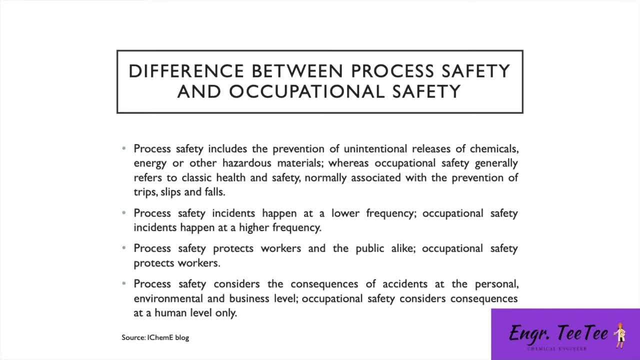 and occupational safety. so the first thing is that process safety involves the unintentional release of chemicals, energies or hazardous materials, while when we are talking about occupational safety, by looking more on things like you know how to prevent trips, slips and falls, and that's so. that's relating to classic health and safety. 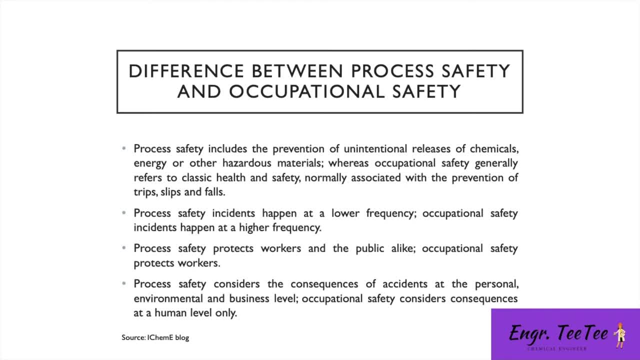 um. so we also tend to see that we have. it's very easy, we have a higher frequency of um, occupational safety incidents. so it's we have higher number of people reporting trips, slips and falls. maybe, you know, even in the office as well. it's possible that you are able to, you you. 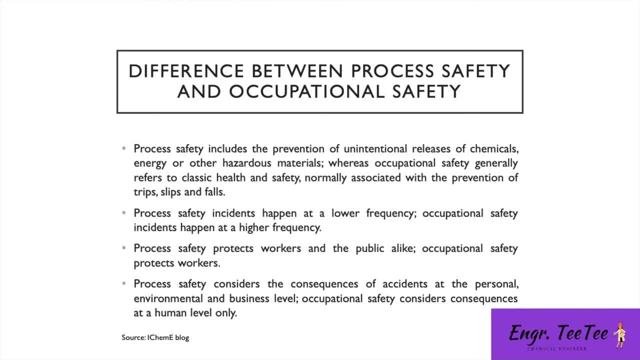 are faced with these things just because you have things all around, as opposed to process safety happening at a lower frequency. so you don't always hear of an explosion every day, or you don't always hear of um. you know um a fire every day as well. um. occupational safety tends to protect. 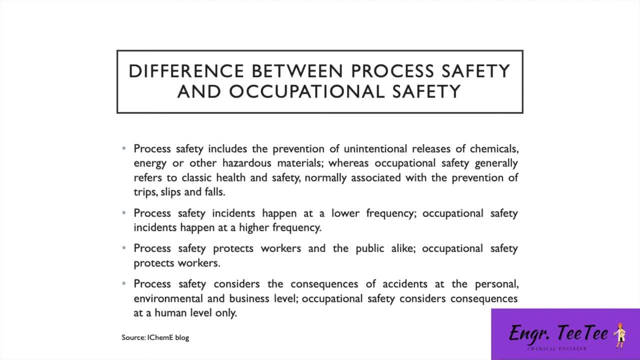 workers, that's, people in the, in the vicinity. so even in the office it's all. the occupational safety tends to involve people around the office, while when we talk about process safety, it could affect the workers and even the public alike. so if we look into the recent um issue, 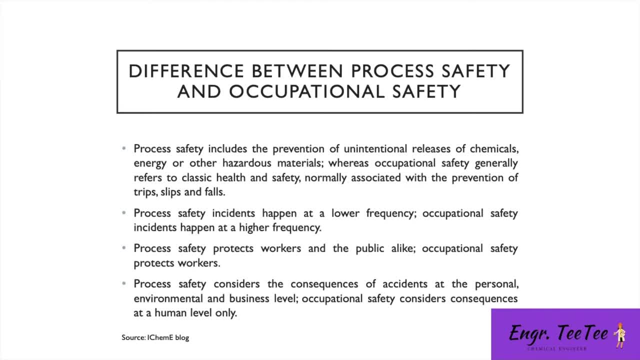 in lebanon as well. so it wasn't just the people in. you know where the explosives were stored. it also, you know, had far-reaching effects, even far into other countries, and the effects were felt in other countries as well. um, the important, another important aspect is that um at process. 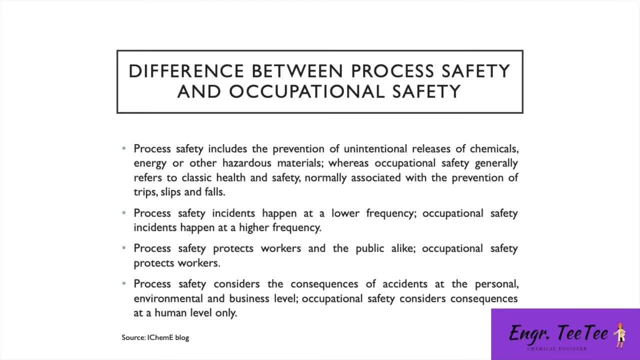 safety. we tend to look at how does it affect the workers, how does it affect the business, how does it affect the environment as well, whereas for occupational safety, it usually- we're usually looking at it as well as the environment as well. so we tend to look at how does it affect the 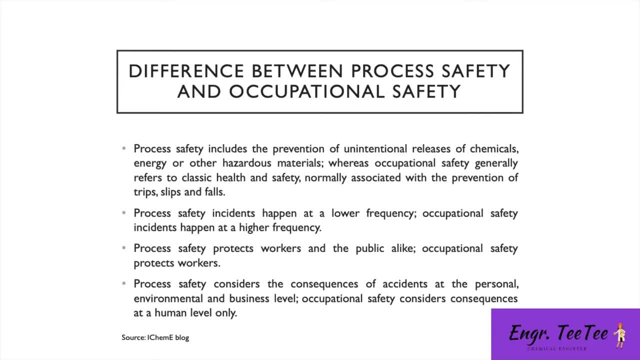 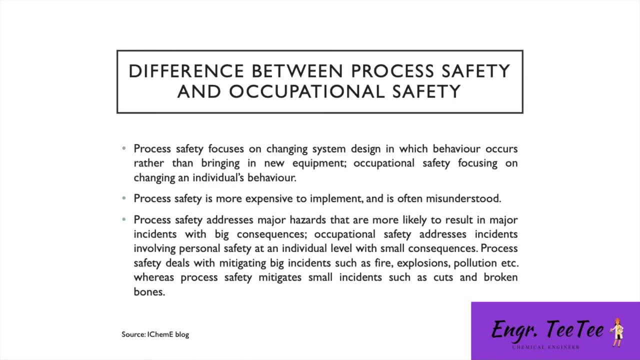 you know, how does it affect human beings um all around in that vicinity? another important part is that while we're looking at occupational safety, we're looking into changing an individual's behavior. so, for example, if we're trying to um prevent an individual from falling from, you know? 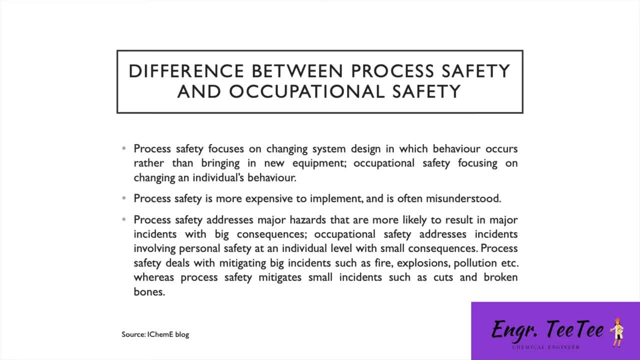 experiencing a sleep or a trip or a fall. well, we're usually saying to people: you know, make sure the surfaces are clean and not wet, make sure you know when you use a tool or you use a particular thing in the office, you know you're not going to fall, or you're not going to fall and you're not. 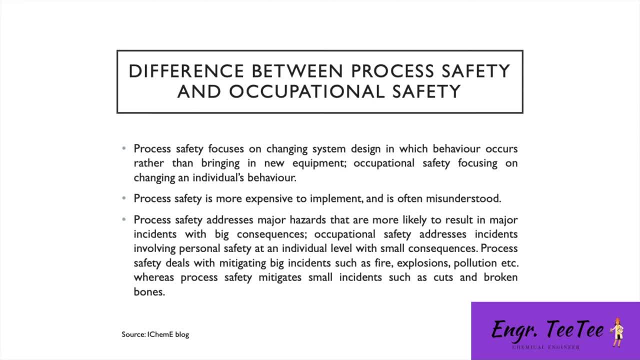 you know you put them in the right place. whereas for process safety, we're looking at changing the system design and um so we, um we're usually looking into changing the system design. we're usually focusing on changing the system design in which behavior occurs, rather than bringing in new equipment, um so process safety is usually more expensive to implement as well. 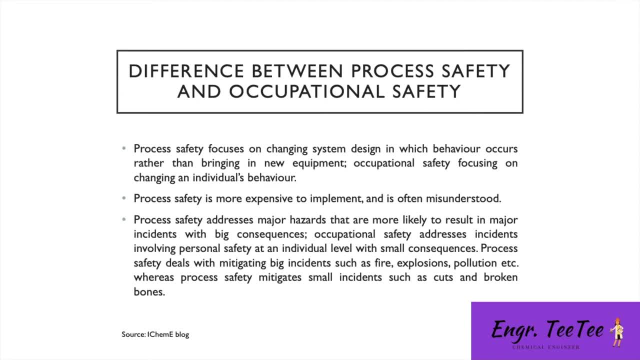 because when you look at things, when you see um, when you identify a hazard, for example, you might then need to put in a fire protection system, whereas for occupational safety, it's more about changing behaviors and, you know, explaining to people. this is the reason why we need to do that um again, process safety tends to have big consequences and major incidents. 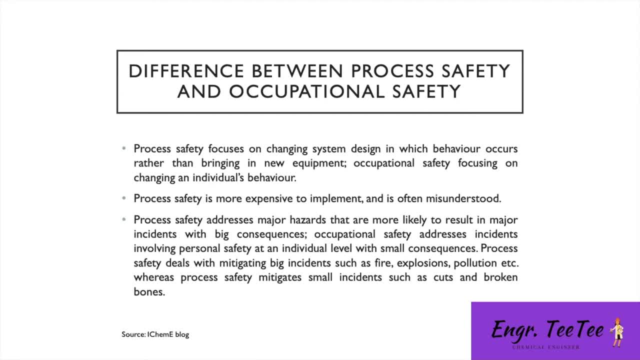 whilst for occupational safety, we tend to see that it's at an individual level, so the consequences are relatively smaller as well. so we're looking more on, you know, cuts and broken bones, which are quite serious as well, but when we compare with, say, you know, explosions, pollutions, fire, um, that's a bigger skill, that's on a bigger scale. 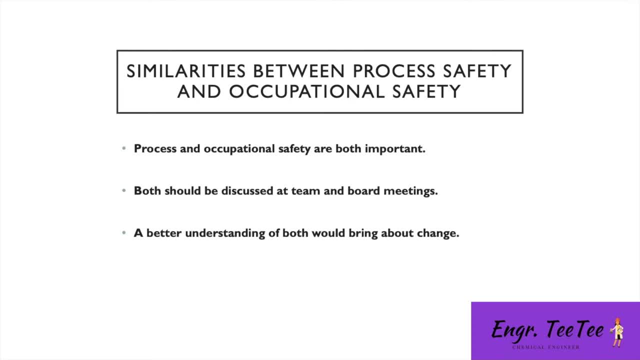 um. but, as well you know, they're both safety, they're both um aspects of safety, and so they are both important. they should both be discussed with different um at both team and board level, and when we understand both, when we have a better understanding of both process and occupational safety, we are able to bring about change in the plans or in the office. 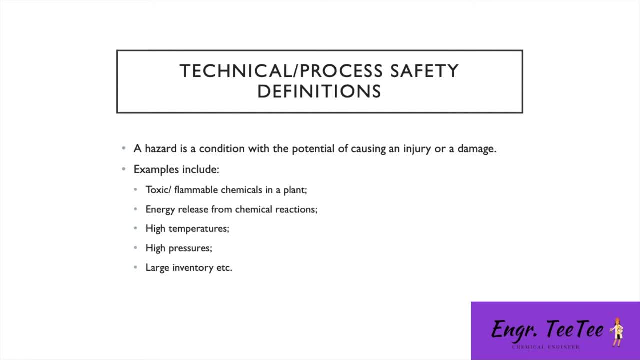 so that's quite important as well. so now we'll look into those things that were highlighted earlier in the video and just try to define what they are. so a hazard is a condition with the potential of causing an injury or damage, so that could be, for example, us having um toxic or inflammable chemical. 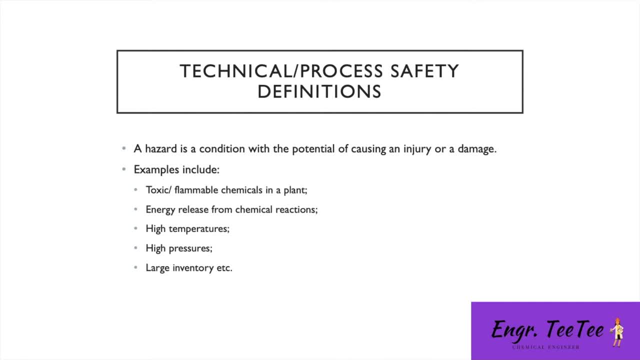 and in their plans. we could also have energy release from chemical reactions. that are the plants. we could have high temperature or high pressure streams, um or fluids on the plants as well, and we could have a large inventory of these chemicals. so these are potential, these have a 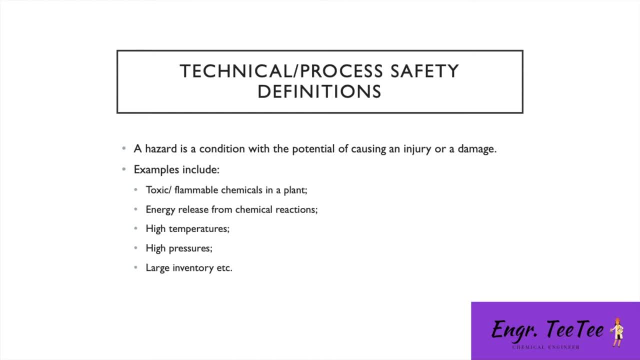 potential of causing an injury or damage in the, with the rights, with the enabling environment present. so when we talk about frequencies- the number of times we have an event occurring in a particular time, or per unit time, and then we talk about consequence, we're looking at what's the measure of these expected effects or undesirable results of an incident, and then 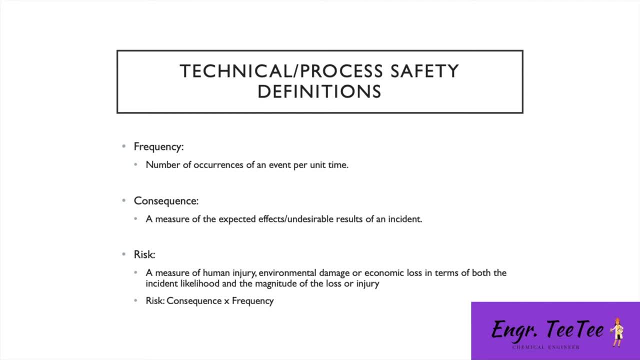 when we bring those together at both frequency and consequence, we then come um, we then end up with risk and that's a measure of, say, human injury, environmental damage or economic loss, in terms of both the incident likelihood and the magnitude of the loss. so, like we mentioned before, 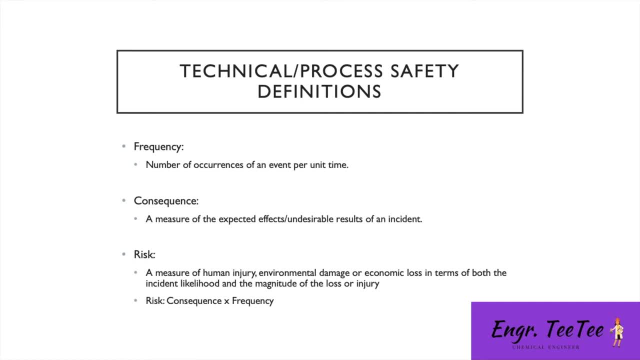 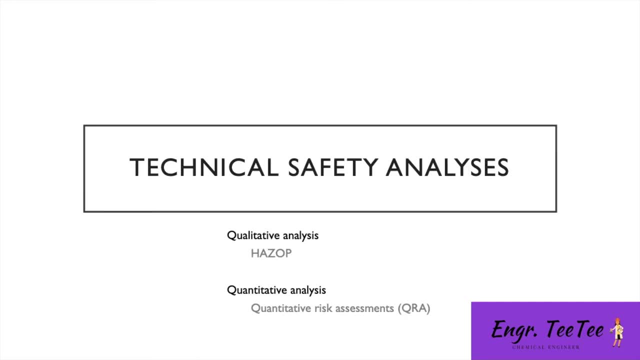 you know, process safety is at human level, environmental level and business level as well. so we could be, we need to look at the risk at those um in those different sectors as well. so now we'll just look into how we do analysis, both from a qualitative and quantitative point of view. 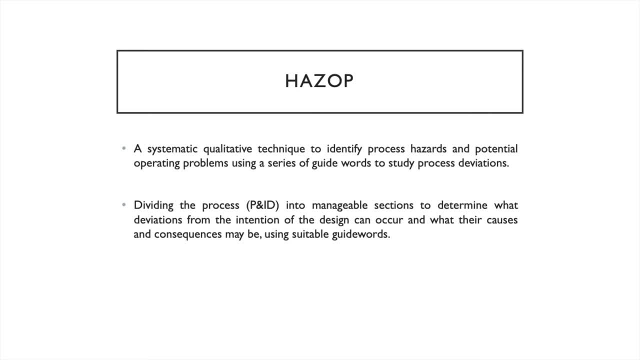 so for the hazard um, that's a hazard and operability study. that's what it stands for and it's a systematic qualitative technique that we use to identify process hazards and potential operating problems, using a series of guide words to study process deviations. so what we do usually is to divide the process, and this could be the um, piping and instrumentation. 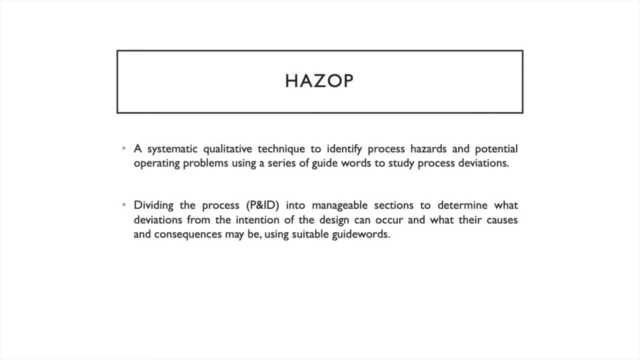 diagram. we're dividing that into manageable sections and what we do is in those sections- or nodes as we call them- we determine how the process works and then we look at what deviations from the intention of the design can occur. what are the cause, what could cause that and what? 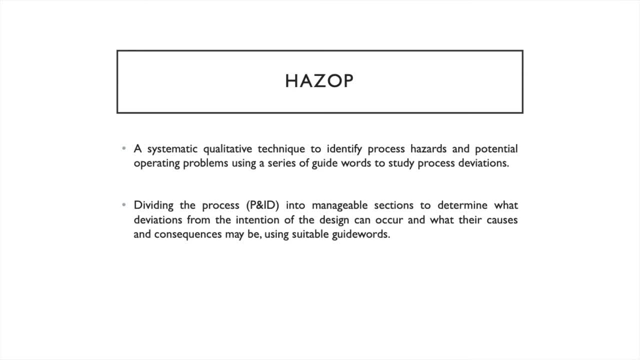 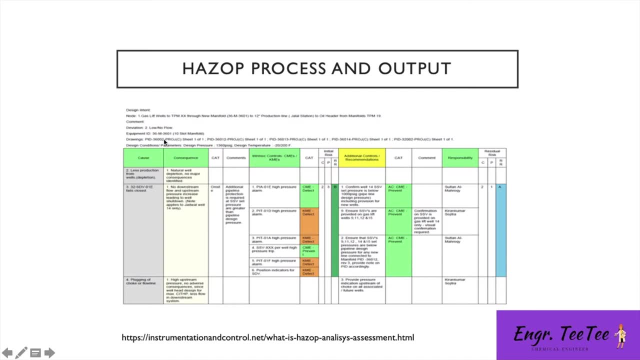 could the consequence be using suitable guide words. so this is an example that I've got from the instrumentation and controlnet website. here we can see some information. so the information includes the description of the node, the design intent. so what is that node supposed to, what is it designed to do? and we have space for comments. 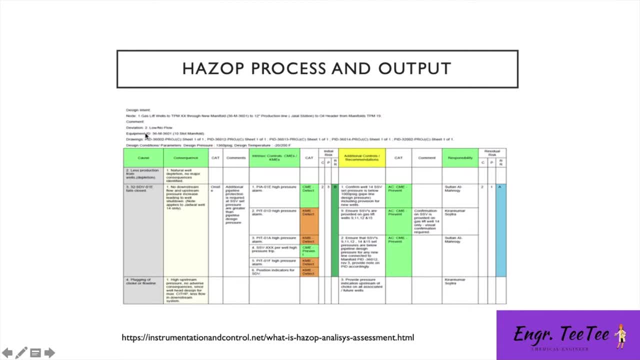 which, if required, and then deviation as well. so in this case, we are looking at if there is low or no flow in this node. we've got an equipment ID as well, we've got a drawing number and we've got the design conditions and parameters in terms of the pressure and temperature. so what we do is: 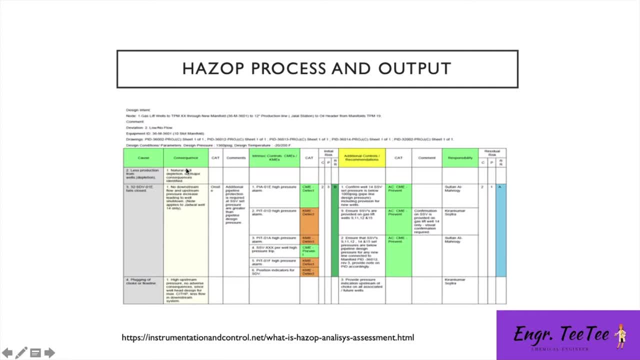 to then identify the cause and then what then happens? as a result of no flow, which is the consequence, we can also categorize these hazards as well, and then if we've got any comments, that can also go in there, and then if we look here, we, as you can see the 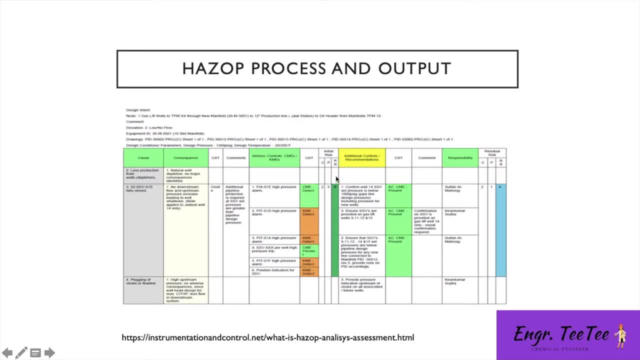 consequence, the probability and the risk ranking. so this is basically how this risk is calculated. so we'll have a look at a risk ranking matrix on the next slide that shows how this is calculated. but this is: this gives us the risk ranking and the color. the coloring gives us an idea of how. 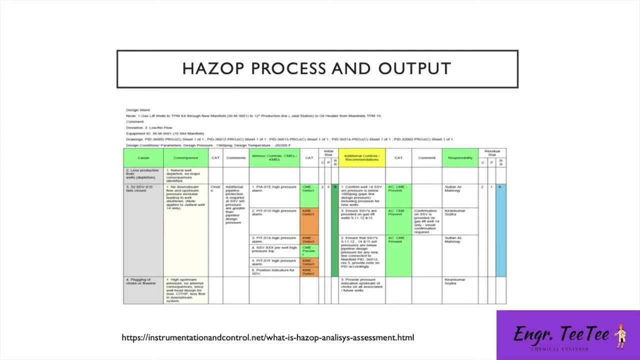 highly ranked or low, low rank, the, the, um, the hazard is. then we've got a column as well where we can identify any additional controls, because what we've done previously is to identify the intrinsic controls, that's, the, the existing controls that we've got, and then, um, we also 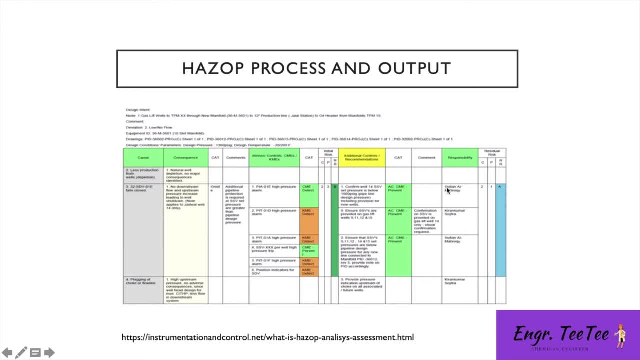 put a responsibility um column for what needs to be done, what additional controls need to be put across, and that's what, that's how we um derived action list. and so we also see a residual risk um column here with the consequence and probability and the risk ranking, and this is 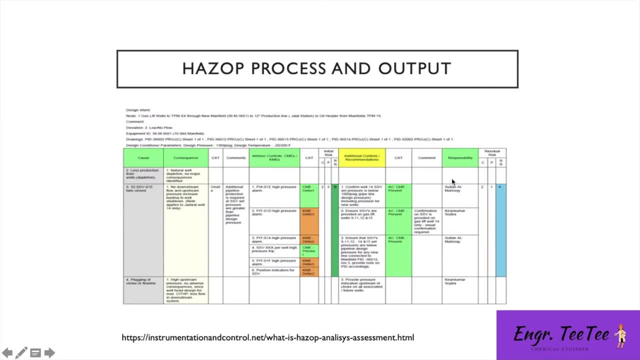 quite important because what we can see is that, after the um application of the additional controls, we can see that the probability of this risk occurring is has gone down from three down to one, and the risk ranking has gone from B to A, which is the um. so this is the goal of the hazard of the 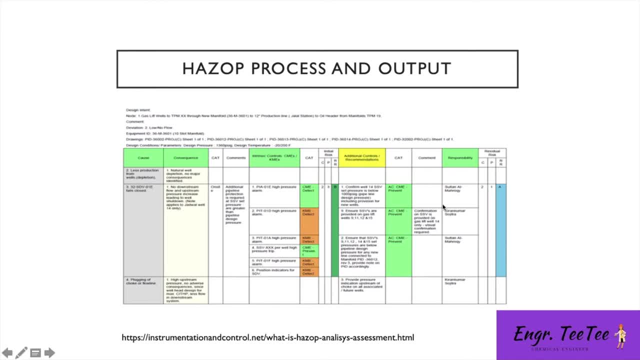 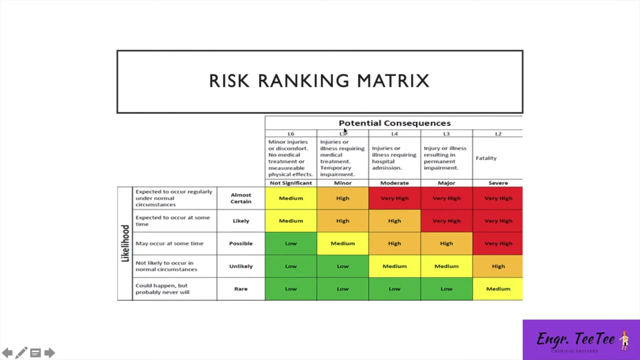 hazard, so we can identify which hazards and to make sure that we also identify mitigation measures to bring them as low as possible, to bring the the risk of the hazard as low as possible. so here we look at the risk ranking Matrix and so- this is quite because it's a qualitative analysis as well- we 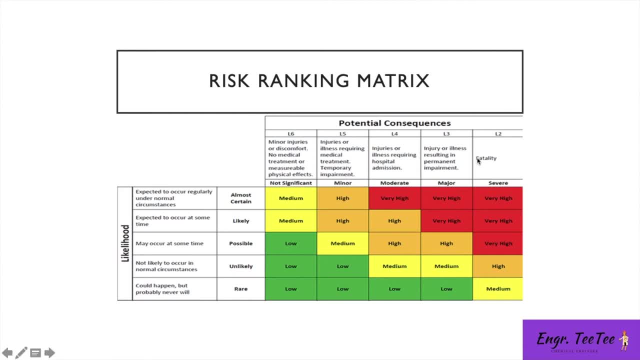 have different bands, so we don't necessarily have to know exactly what the consequence is in um numerical values where we can identify what band it is we are. what we are saying is: if we get a risk, um, so if we get a hazard actually occurring, what's? 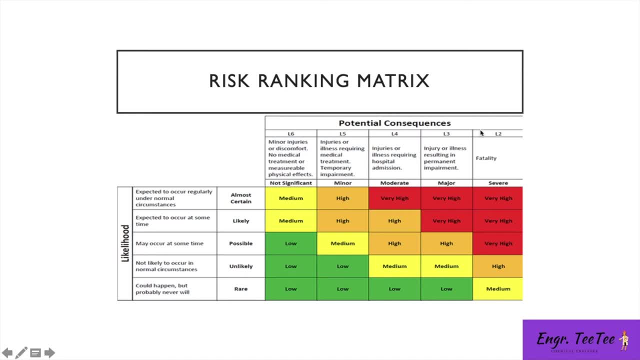 the consequences of that. is there going to be minor injuries or is there going to be a fatality? so if we're able to you know what we we aim to do during has ups is to identify which band that occurs, the hazard occurs. what we aim to do in hazard- hazard, what we aim to do in has ups- is 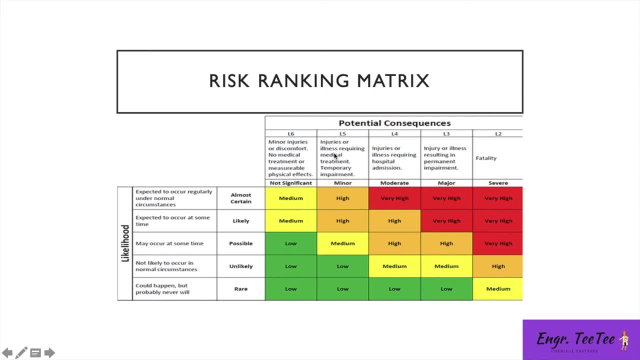 to identify the consequence um band and then um place the hazard accordingly in that band. in addition, we'll look at the likelihood, which is what we can see on the horizontal, and again that's trying to, you know, just place it in a range um as opposed to getting an exact value. 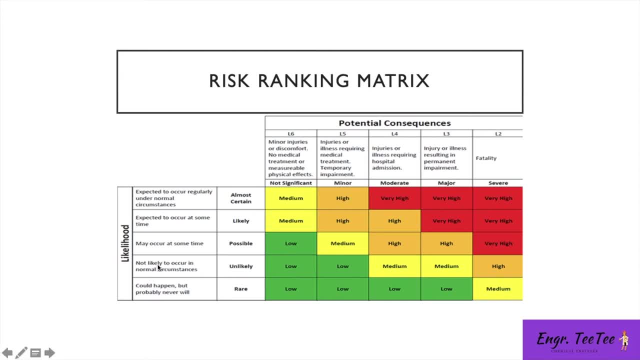 and so when we get that- so, for example, if we've got a hazard that's not likely to occur in normal circumstances, when it does occur it leads to injuries or illness that requires hospital admission- then that has a medium risk, and so what we'll be trying to do is to reduce this, possibly um. 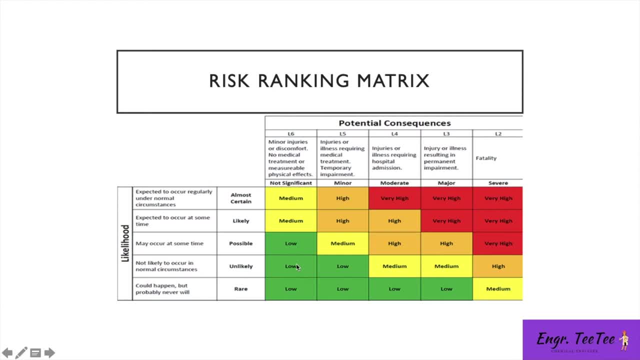 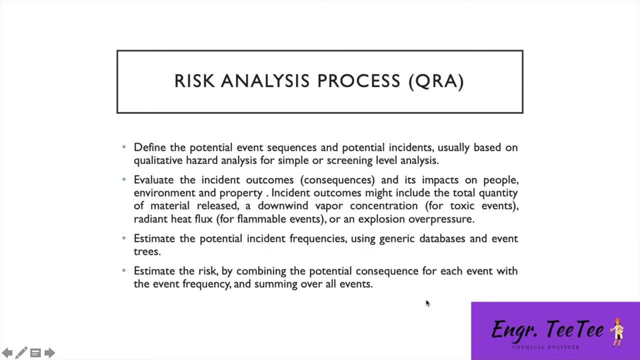 to a low risk or, you know, or low, lowest risk. so we'll be trying to move it this way. so the aim is to move um all the risk as much as possible to, you know, the low risk, um the green zone. so in the quantitative risk assessments what we do is quite similar as well. we define the 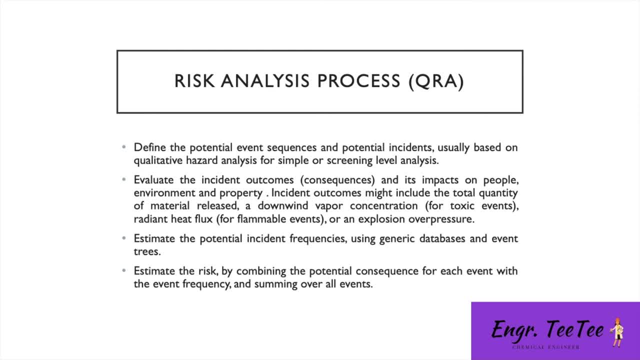 potential event sequences and the incidents and then- and this is usually based on qualitative hazard analysis, um, or initial analysis that we do- and then we evaluate the consequences. we evaluate the impact on people, environment and property and then after that we estimate the potential frequency- and we do that using generic databases and event trees- and after that we 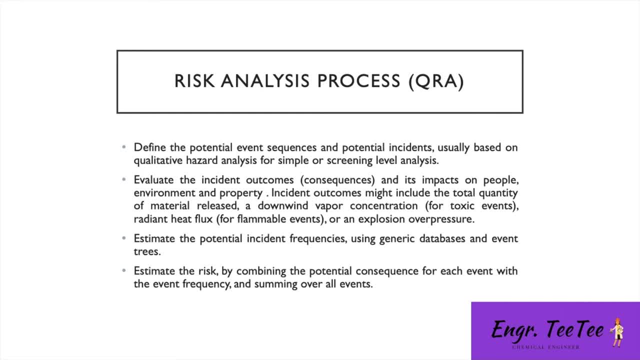 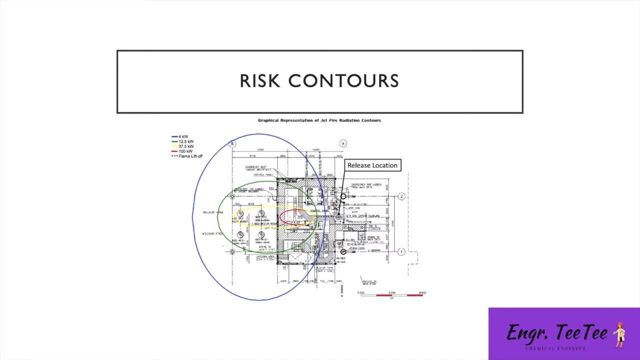 estimate the risk, once again by combining the potential risk, the potential consequence for each event, with the event frequency and summing that over all events. so this is an example of a risk contour we would get using a modeling tool, and so here we can see a release location that this: 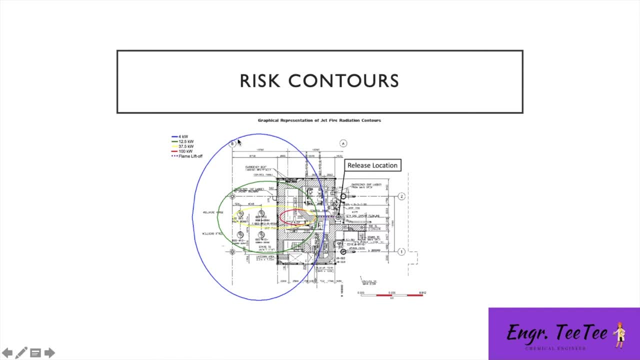 is the area within which, for example, you will feel the four kilowatts of risk. and then we can see the four kilowatts um radiation, um based on a release um from this location. and so this shows this, this shows the risk contour for a single release location, and you can see that this is. 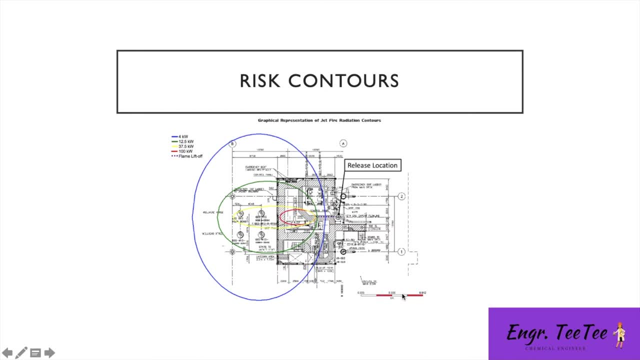 superimposed on a plot plan and we can see here in the plot plan- this is this i got from the of the internet as well- um, this shows the scale, um that has been used for the plot plan. so here we can see the uh, the risk contour and um, you know, you can see the Community. 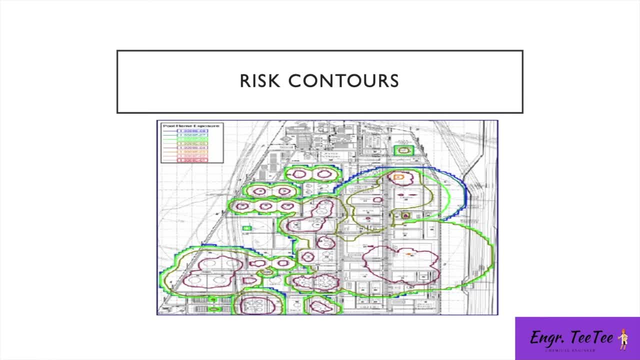 the area in which the effect of the flammable radiation can be felt. so this is, then, what happens. this is another example of a risk contour, but this shows what happens when you know the risk is summed over all events that could occur from different release locations, and so this again is. 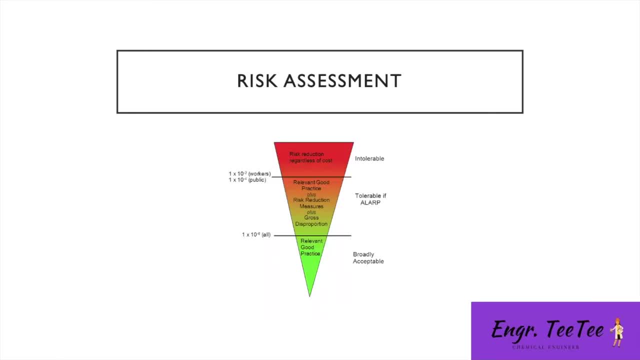 superimposed on a plot plan, and this is an example that i got from the plot plan, so here we can see of the internet as well. so this is an alarm triangle, and what we do is show where our risk lies. so as we, so when we, then when we're able to, so when we sum up all our risk over all events, we 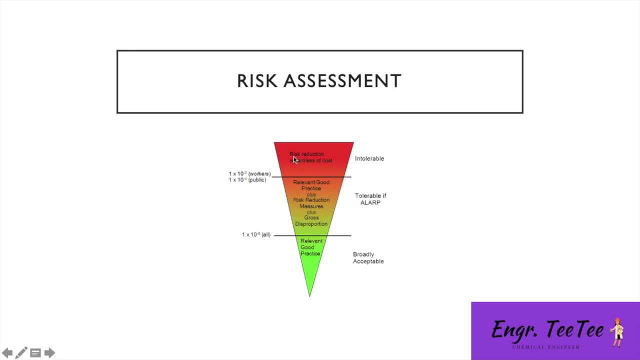 get a single figure and we're able to then realize, pinpoint where that, where the risk lies, whether it lies in the intolerable region or the tolerable if a lap region or the broadly acceptable region. so when we're in the intolerable region, we definitely need to apply risk reduction. 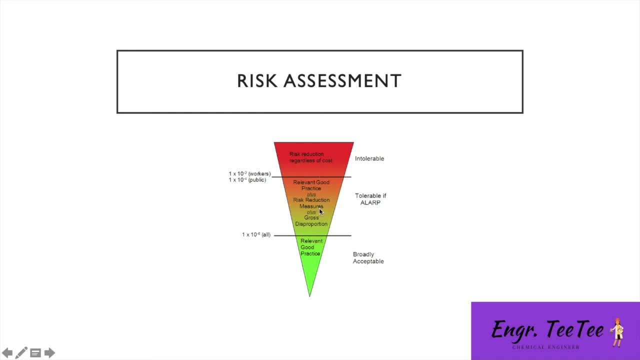 measures to move it into the tolerable if a lap region or the broadly accepted region. if we're in the tolerable, if a lap region, then it means that we can- um, we can- employ relative relevant good practice plus risk reduction measures as long as they are grossly disproportionate, and then if we're here, then we're good. yeah, we can also. 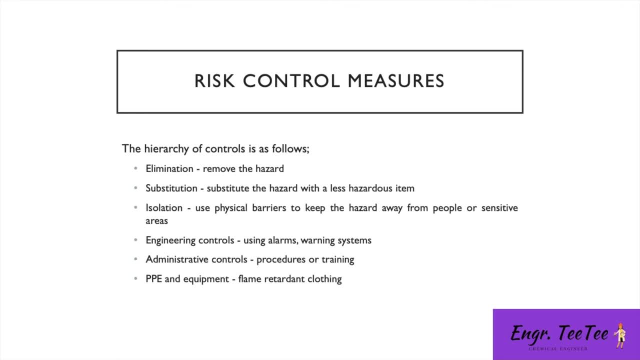 see that we have different risk levels for workers and the public. so I'm talking about risk control measures. the hierarchy of controls is to try to eliminate the hazard. if we can, that's to remove it, we can then try. next, we try to substitute the hazard with the less hazardous item. if we can't, we 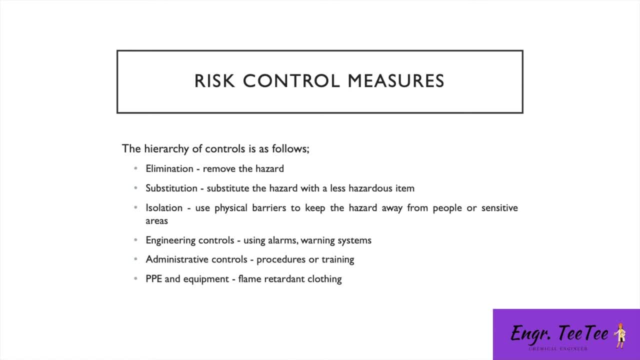 try to isolate it, which is to use physical barriers, and then we can then try to remove it to keep the hazard away from people or sensitive areas. so an example of this is applying a bond around a place where we know that we can leak, say, flammable material that can turn into a pool fire. 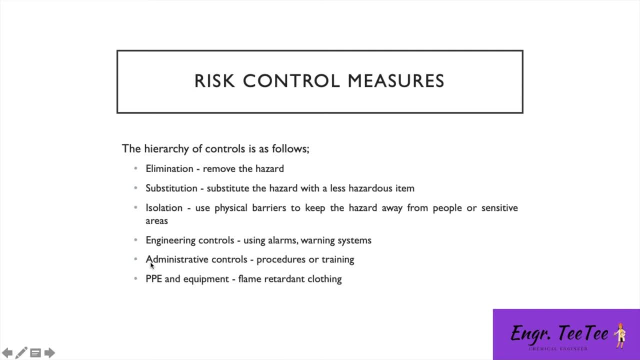 for example, and then next we look into engineering controls, that's, using alarms or warning systems to alert the operators, to know what to do next. if we can't do that, or in addition, we can put in administrative controls, which are procedures or training of the operating staff as well, and then 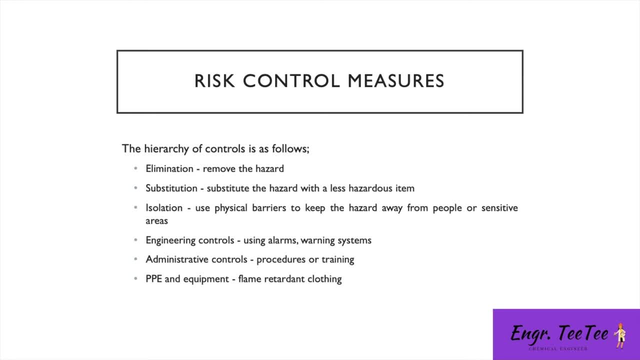 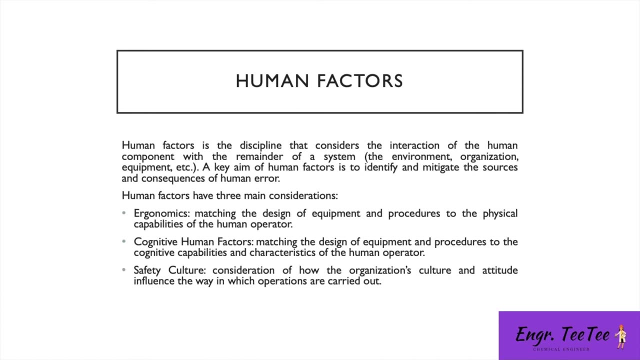 we provide personal protective equipment and other equipment to ensure that if there is an explosion or a fire, there's, you know, there's personal protective equipment to guard against that, but that's always the last resort. the next thing we need to consider is human factors, and this is. 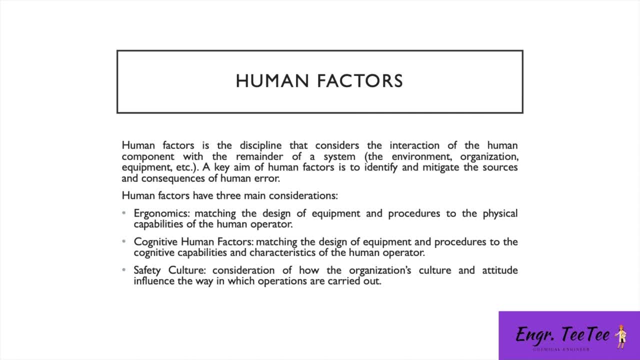 important because we are in a situation where we are in a situation where we are in a situation where we are considering, we need to consider the interaction of the human component with the actual system, and one of the things- and these are- this can be divided into three things. so ergonomics, and that's. 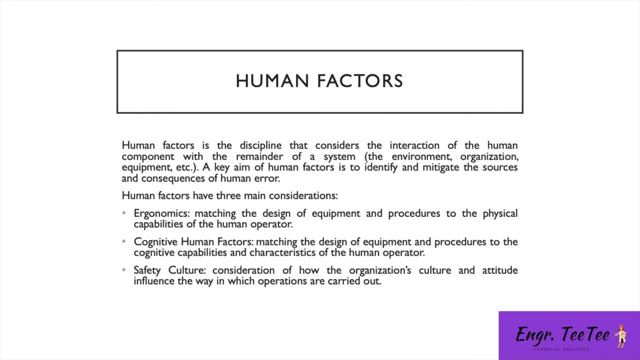 this. what that entails is matching the design of the equipment and the procedures to the physical capabilities of the human operator. the next thing is the cognitive human factors, and that in that case we are matching the design to the abilities and the characteristics of the human operator. and then safety culture as well is quite important, because this is- this is more on an organizational 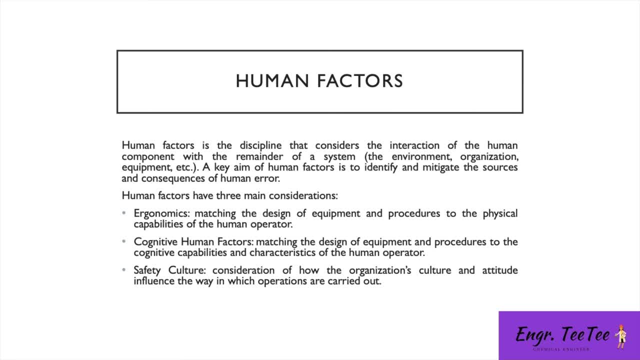 level, just trying to understand and make sure that the the organization has a good culture and good attitude that influences the way operations are carried out, and this includes things like how, how often do we check our safety practices? what happens? what's the procedure? what if someone identifies something that is something that is problematic? or if you identify something that is? 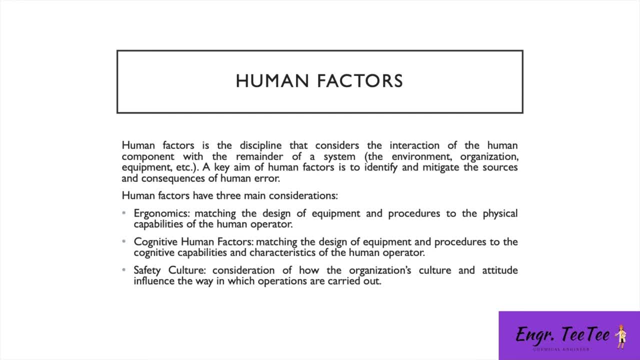 something that is problematic, then you can attack that person. it is very important because if there's not unsafe, is there, you know, is the person, is the person which hunted or you know, is the person sort of allowed? are people allowed to express themselves freely when it comes to safety as well? 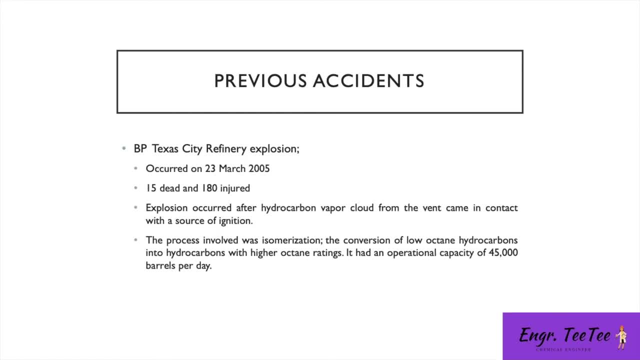 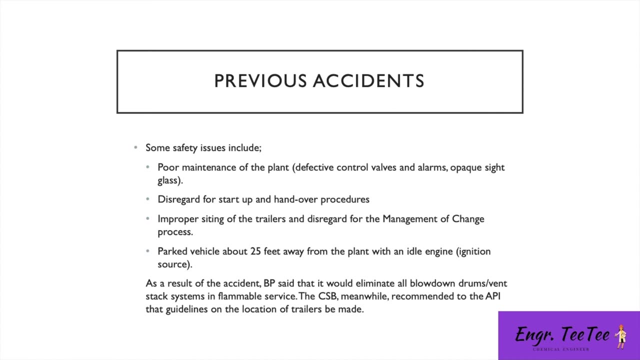 so these are things that need to be considered. so, if we look at previous accidents, we have accidents such as the texas city refinery explosion that occurred in 2005. we also have and, and here we can see that some of the safety issues were, you know, having to do with start-up. 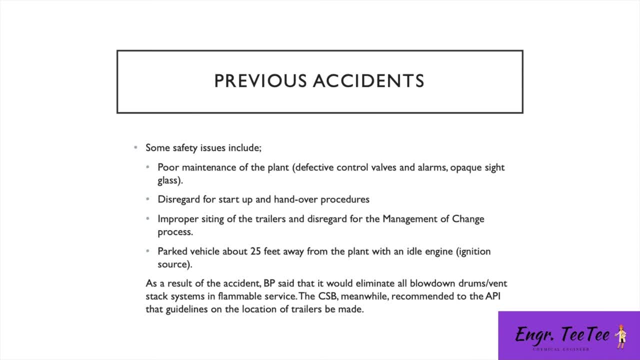 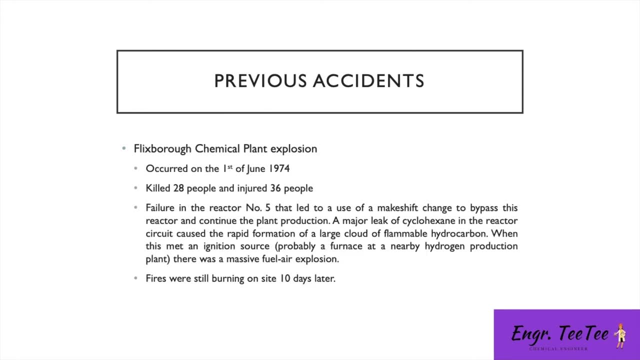 poor maintenance, improper sighting of trailers and um the presence of an ignition source. another accident was in 1974, which was the flixborough chemical plant explosion and that was a cyclohexane plant and it was quite serious because the fires were still seen. 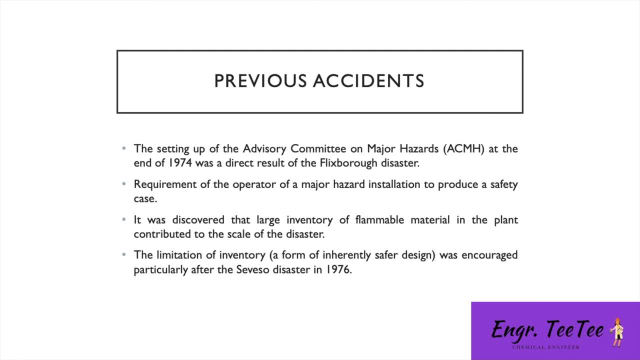 but this was quite um an important part of history because, in addition to this and to the flixborough accident, as well as the cervezo disaster in 1976, the main thing that came out of those is the fact that, um, there was a limitation of inventory, that was encouraged.